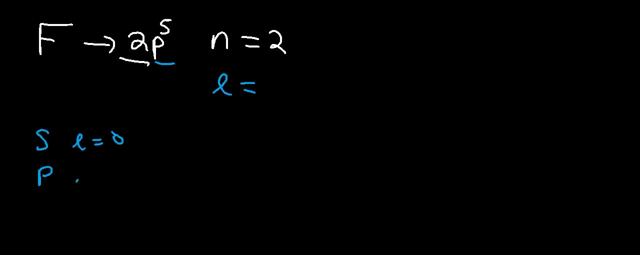 For S, L is 0.. For P, L is 1.. For D, L is 2.. And for the F subshell, L is 3.. So therefore, L is 1.. Whenever L is 1, you know, ML can be these three values. 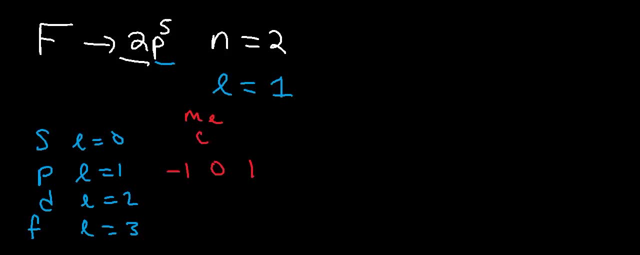 Negative: 1.. When L is 0, ML can be 0.. When L is 2, ML can be these five values. When L is 3, ML can be seven possible values. The values for ML corresponds to the orbitals of, you know the sublevel. 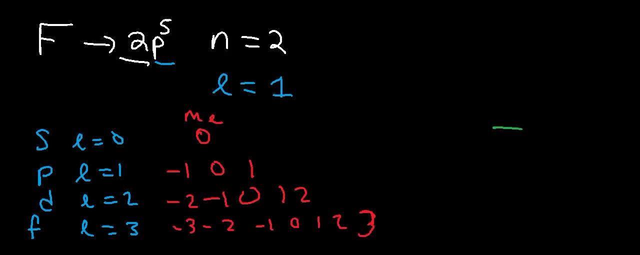 S only has one orbital because S can hold up to two electrons. Every orbital holds a maximum of two electrons. P has three sublevels, D has five, F has seven, And each of these ML values corresponds to a certain orbital. So since L is 1, ML can be three values. 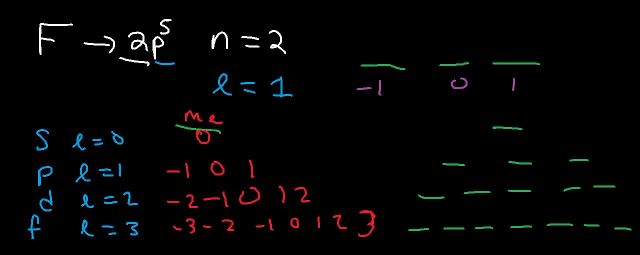 It can be negative: 1,, 0, or 1.. Now we're dealing with the fifth electron, the 2P5 electron. So 1,, 2,, 3,, 4, 5.. That's the electron we'll focus on. 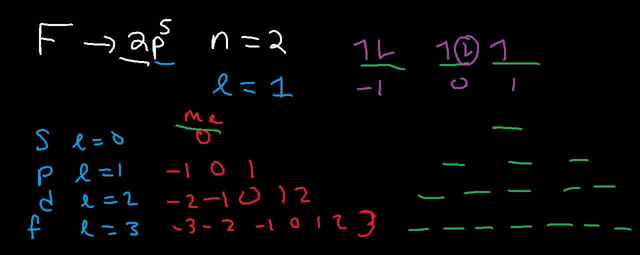 So that electron landed in the 0 orbital. But none of these numbers areutive for ML. So therefore ML is equal to zero And MS the electron spin. because the arrow is facing downward, it's going to be negative 1.5.. 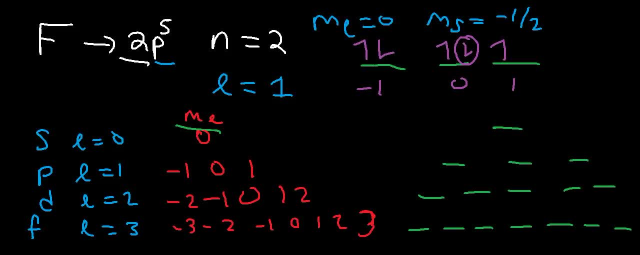 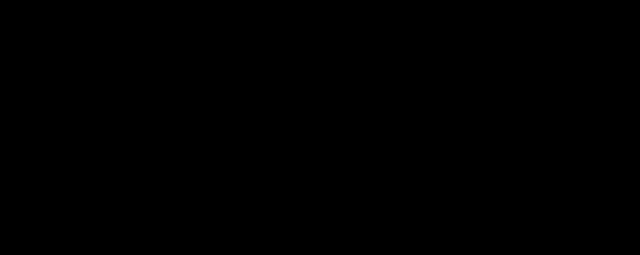 So those are the four quantum numbers for the fluorine atom. the last electron in the fluorine atom, the 2P5 electron. Alright, let's try another example. So let's say if we want to find the four quantum numbers for iron. 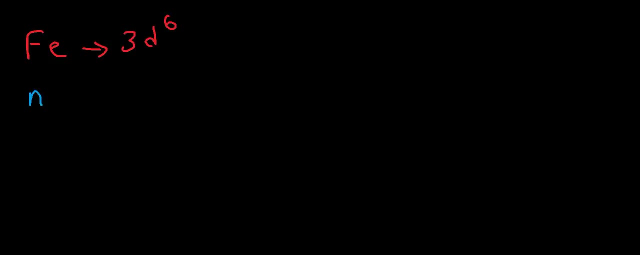 electron. well, we know n is 3 because you know that number. it's in the third energy level. for the D sub level, we know L is 2, remember. for S it's 0, for P is 1, for D it's 2, for F is 3. now the D sub level has 5 orbitals and ML can be, it can vary.